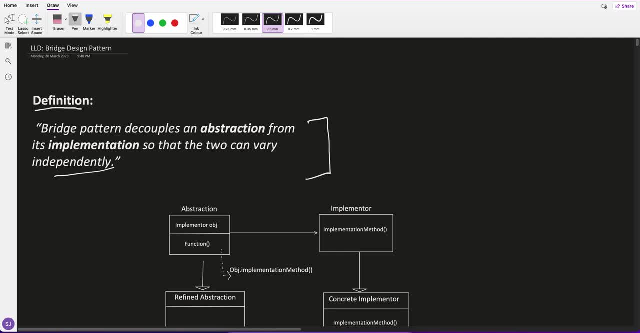 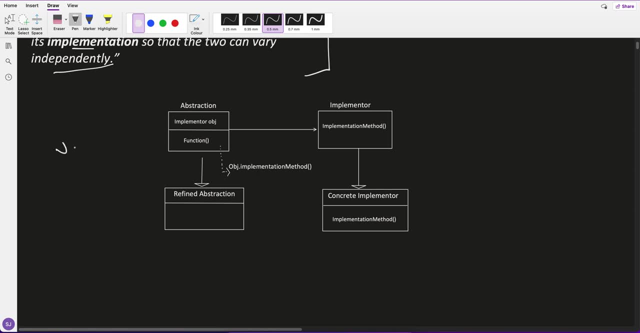 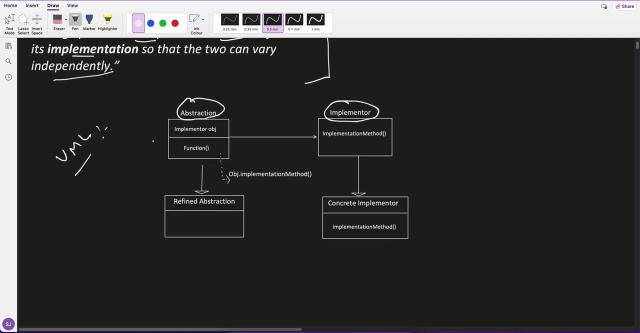 get clarified with this definition very easily. So read one more time: Bridge pattern decouples what abstraction from its implementation. So this is its UML, So this is abstraction. This is implementer Right. So it decouples an abstraction from its implementation so that two can vary independently. So let's say: if you want to increase more concrete implementer, you can add it here. 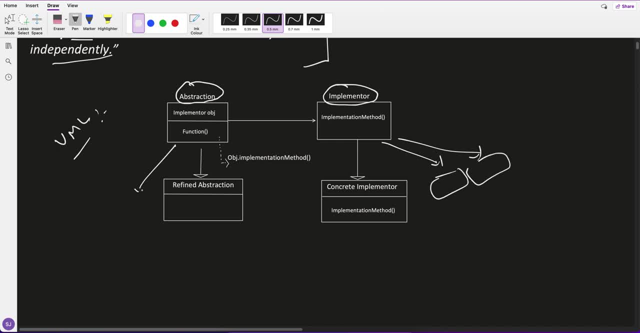 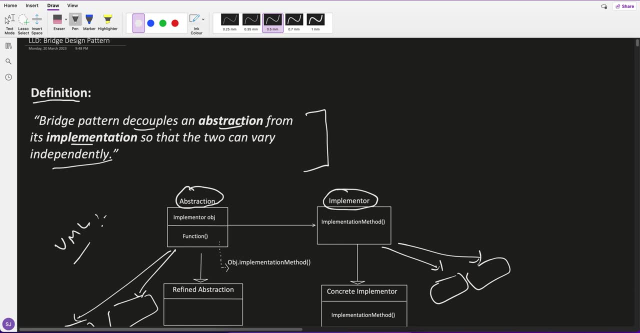 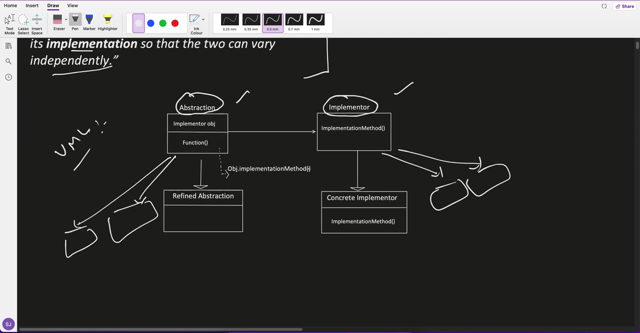 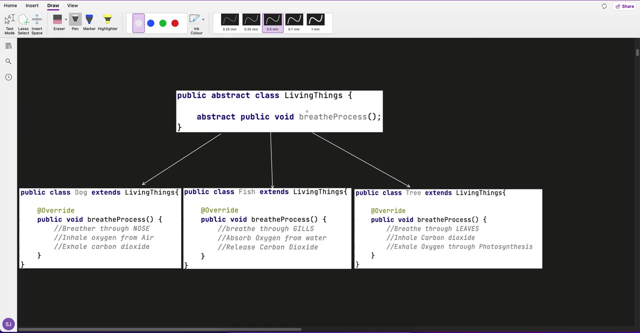 If you want to add more child classes for this abstraction, you can add here. So that's why I say that it decouples an abstraction and implementation so that they both can vary independently. Right, We will come to this UML again, but let's see first an example and understand this definition properly. So I come up with an example. is this: let's say: living thing Right. What living thing? Right? So I come up with an example. is this: Let's say living thingurosưaada. So I come up with an example. is this: Let's say: living thing Right. What living thing right? What living thing? 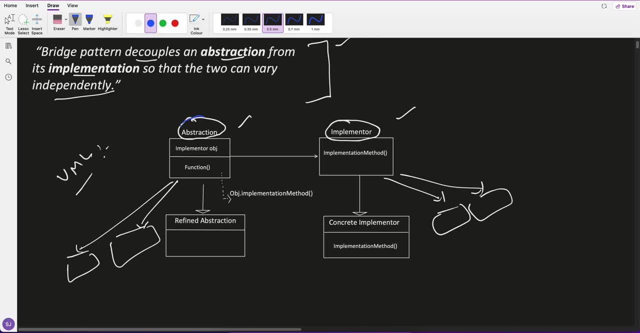 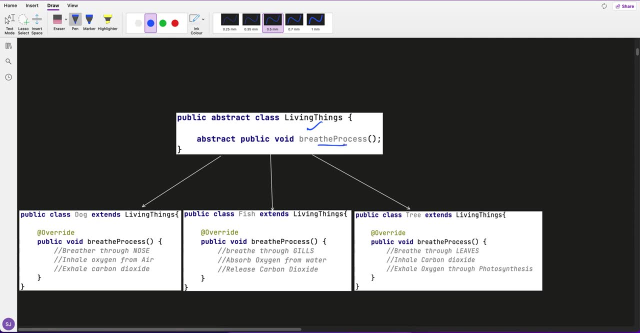 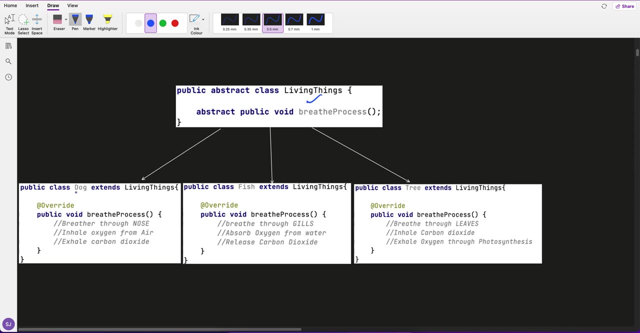 so this is an abstract class, this one, this is an abstract class, right? so here i have created one abstract method: breathe process, breathe process. so now i created a three child classes- dog, fish and tree right- and i have a breathe process method. so it's a abstract method, right? 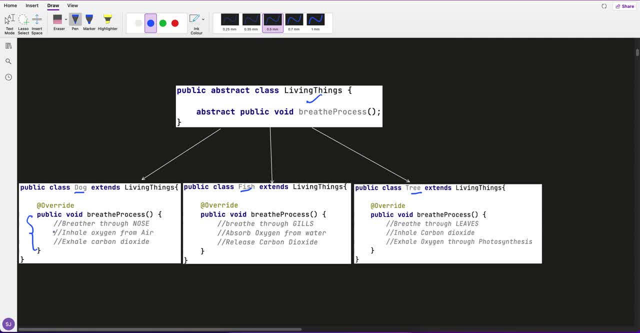 so they have to implement it. so if you see that dog has its own breathe process, it breathe. so it breathe through nose, inhale oxygen from air and exhale carbon dioxide. similarly, fish has its own breathing process. breathe through grills, absorb oxygen from water, release carbon dioxide. tree. 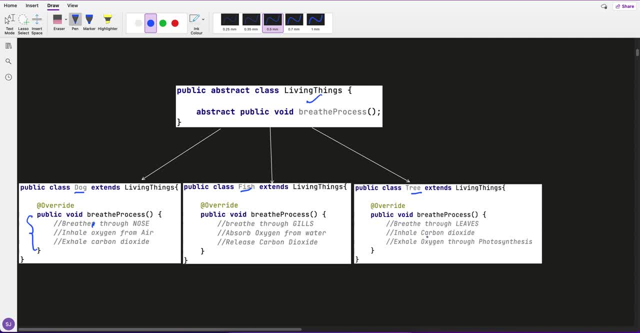 has its own breathing process: breathe through lips, inhale carbon dioxide, exhale oxygen. okay, so now, if you see that this is nothing but a simple inheritance inheritance, you will say: this is nothing but a simple inheritance, right? so the parent class has this method and all the child class just implemented those methods. but what is the? 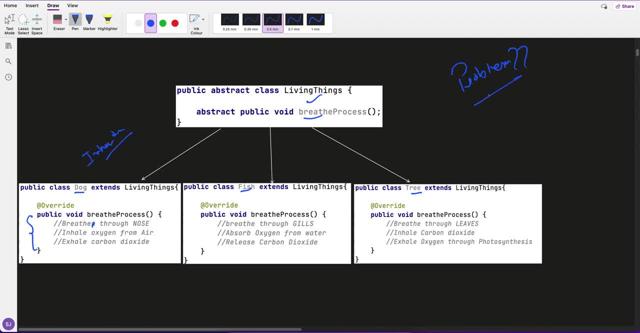 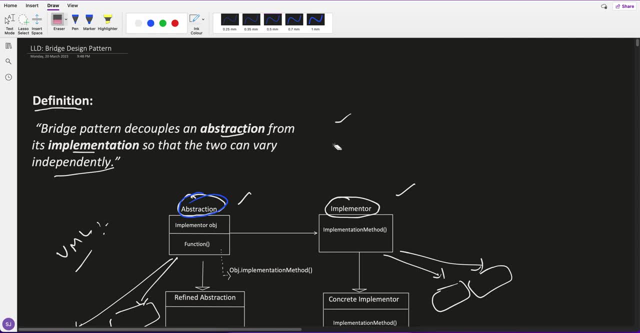 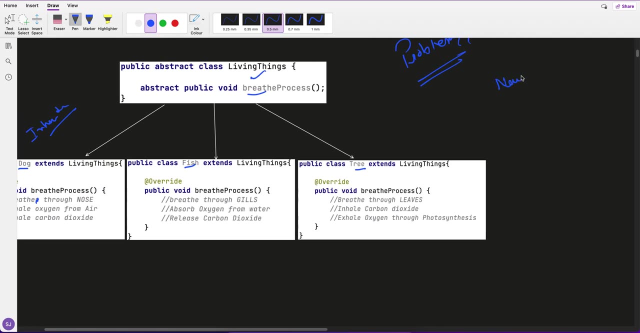 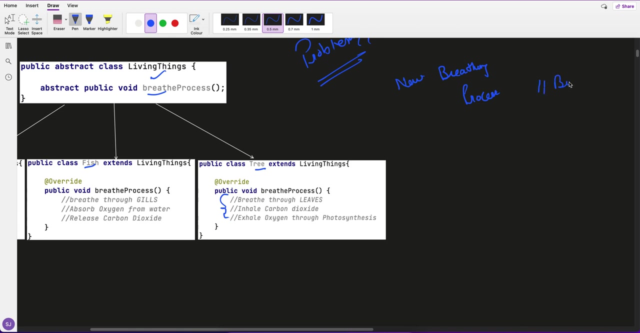 problem here? what is the problem here? right, which bridge pattern is trying to solve? now we will see the problem: which bridge pattern try to solve in this thing? okay, so here the problem is. now, let's say: I want to introduce new breathing process, new breathing process, so this is a process. right, let's say, I want to like breathing process, let's say for bird. 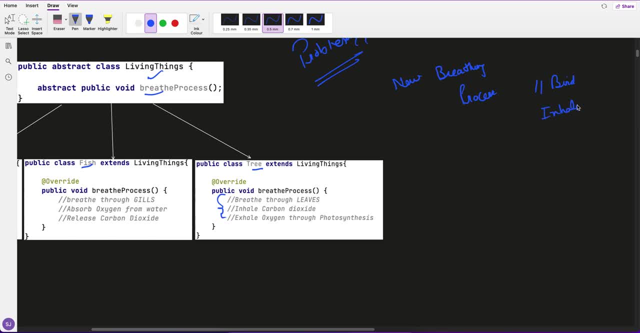 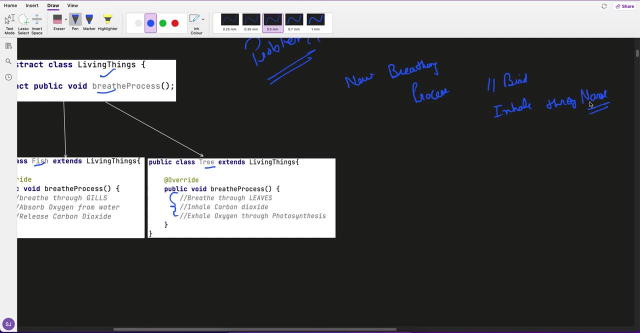 let's say bird breathing process, is it inhale through nuts like they have a beak, and on the beak they have small holes. So that's called breathing process. So that's called nuts, right? so let's say they- now it's a different breathing process- inhale. 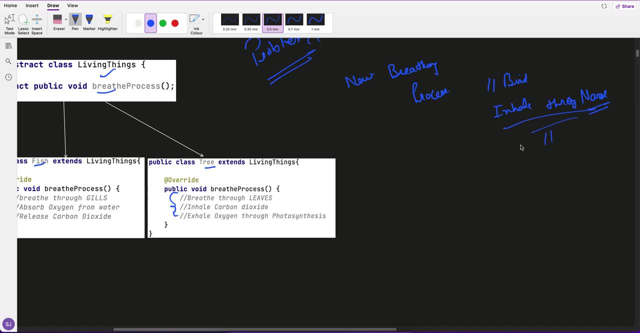 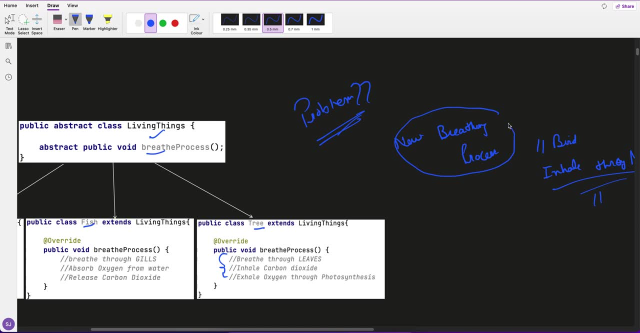 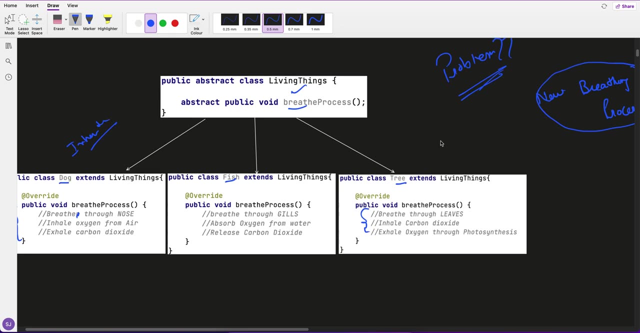 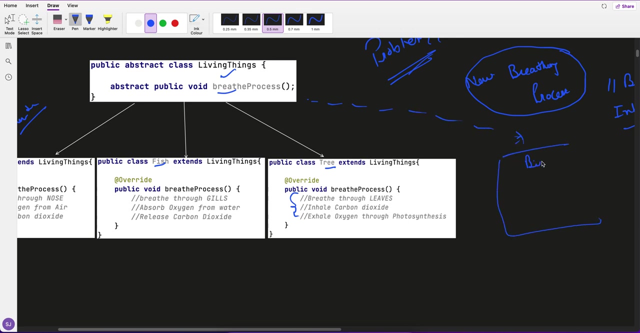 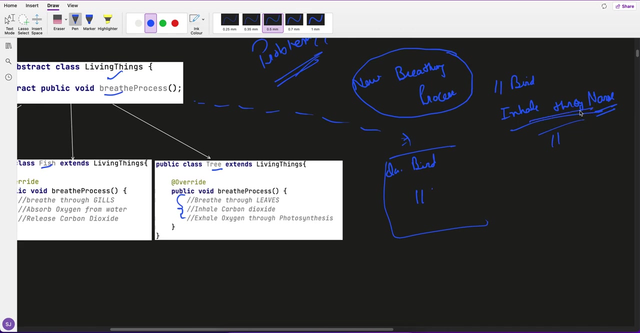 oxygen, exhale carbon dioxide, so it's a different breathing process. now the problem here is you cannot add this new breathing process because currently it is very tightly coupled with the abstraction. so until, unless this will not add bird right, So another class. but then only you can add this breathing process: inhale through nuts and exhale through mouth. let's say breathing process something. 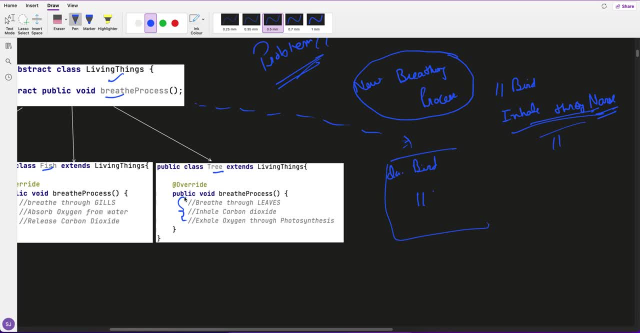 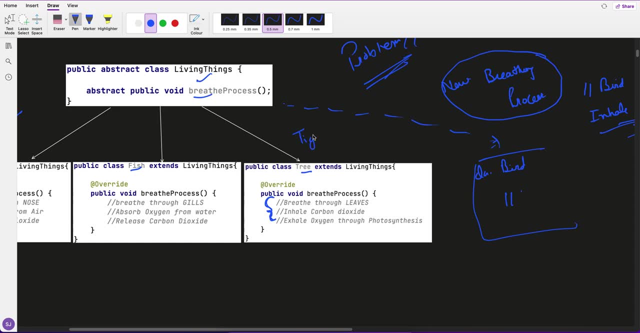 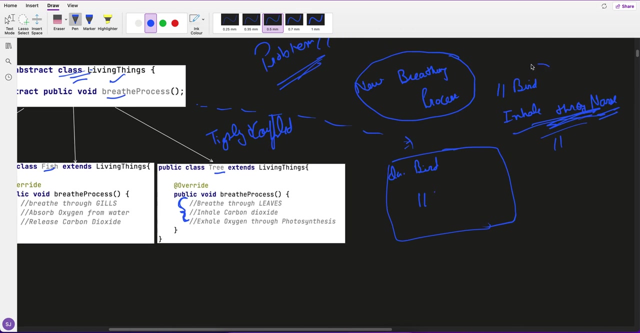 So what I'm trying to say is that here, even if you wanted to add a new breathing process, you cannot add it because it's very tightly coupled here. tightly coupled With what? With abstract class. until, until, unless, As abstract class is there is no child class present which use that breathing. 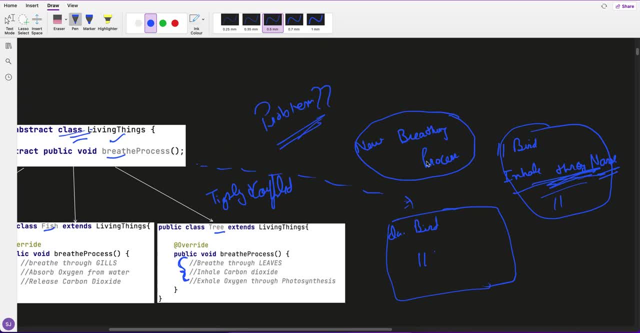 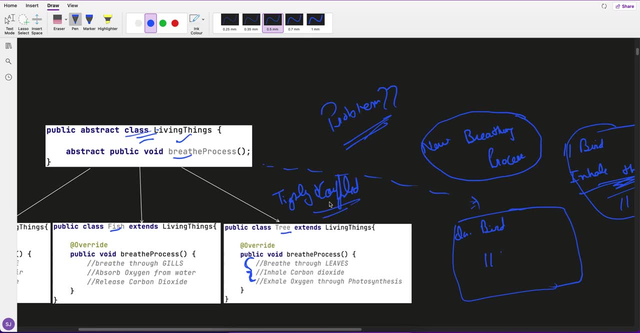 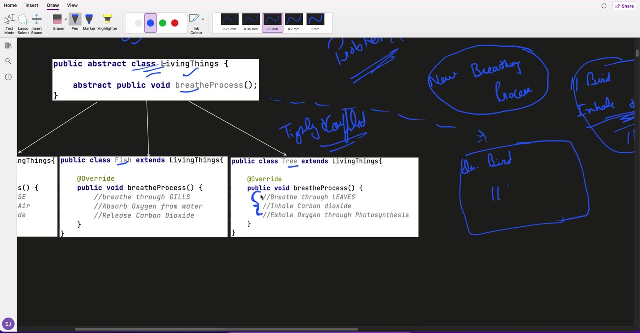 process. you cannot add it right, so they cannot vary independently. they are very tightly coupled. you understand the problem, right, you got it. so the problem here with this example is very clear. right, if you want to add a new breathing process, let's say anything. right, somebody inhales, let's say something. 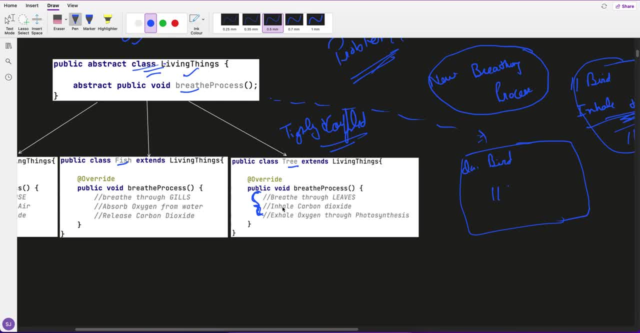 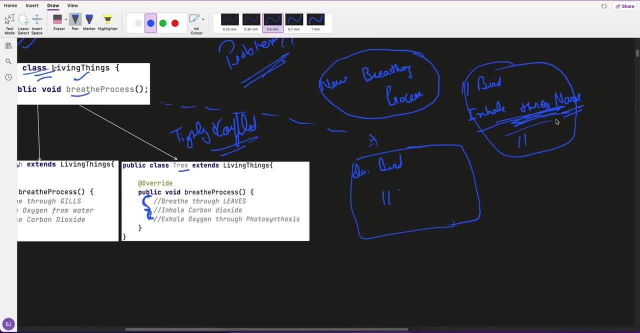 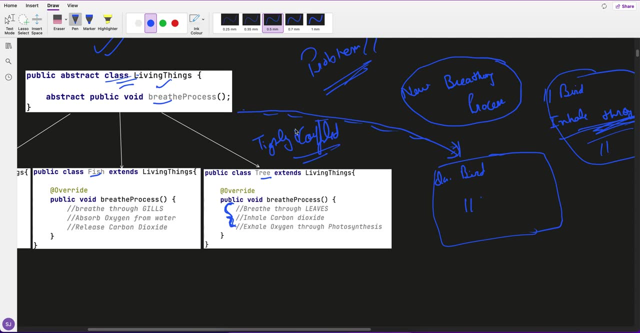 carbon dioxide and leave and exhale also carbon dioxide- both inhale carbon dioxide, exhale carbon dioxide. so it's a totally different process, right? but you cannot add it unless and until an unless there is one child class added into this abstract which uses that, which uses that breathing. 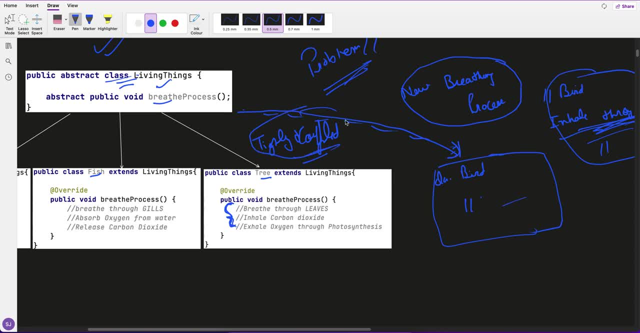 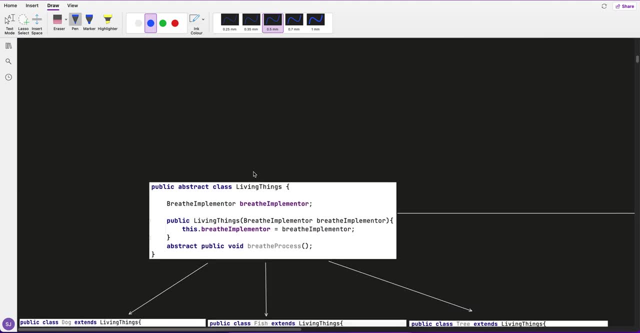 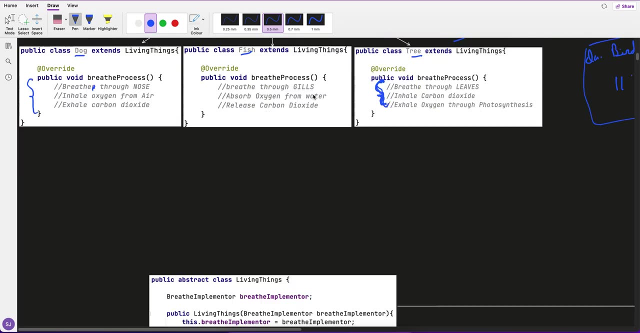 process. so why? because it's a tightly coupled this implementation and abstraction. so how to resolve this? so I have divided into this part. so what I have done is so living thing: I have maintained the same thing, abstract class, living thing, right, but what I have done is I have 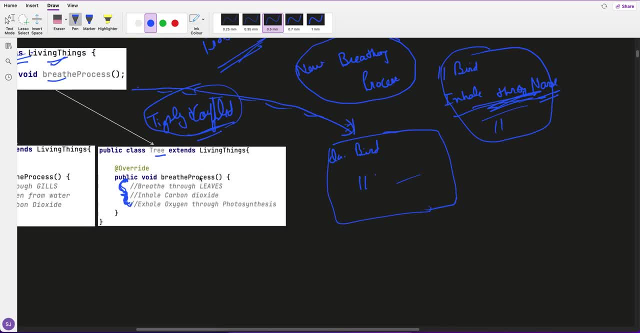 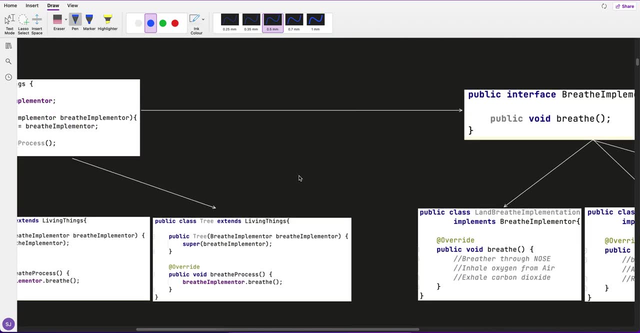 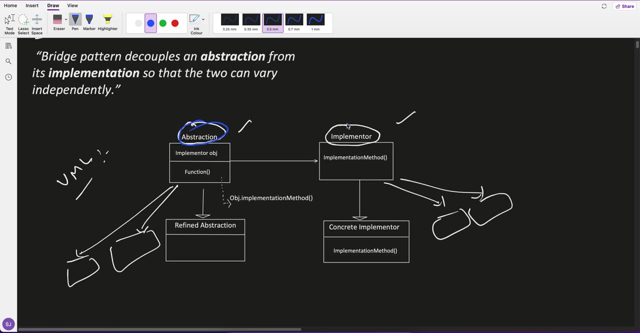 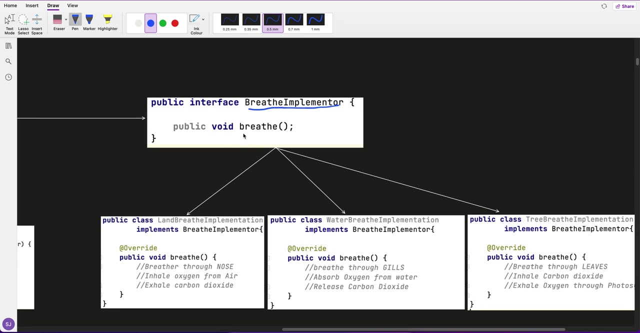 taken out: the breathing. this is right. I, this process, this implementation, breathing process, I have taken out in a different interface. so I have created one breathe implementer. so I have created one implementer which is known as breathe. I given a name: breathe implementer, right, so it's is. it has one method: breathe. it's an interface. now I've created a child glasses. 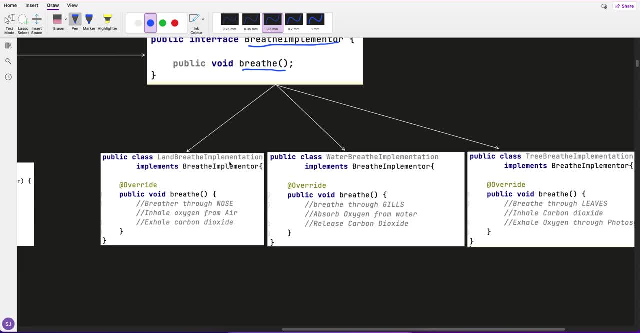 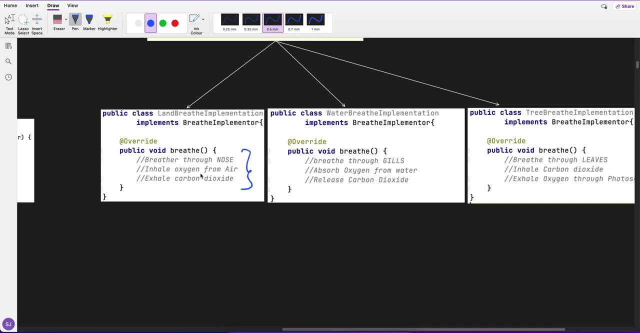 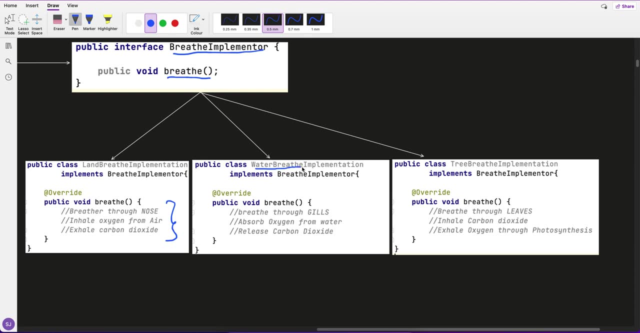 I end with the different processes. land breathe, so I give it a name. land breathe, so it's has its own implementation. okay, breathe through nose: inhale oxygen, exhale carbon dioxide. similarly, i have created one child class: water breathe implementation. breathe through gills: absorb oxygen release. 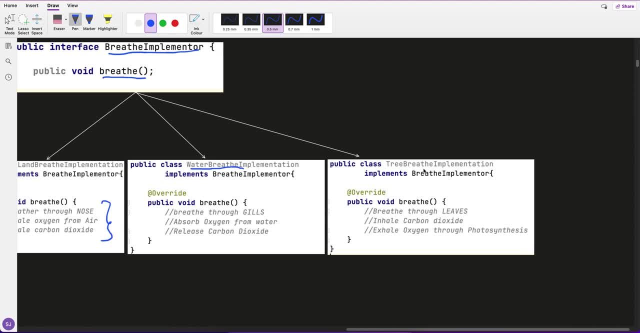 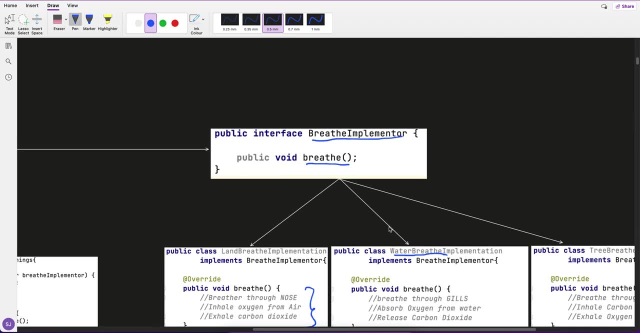 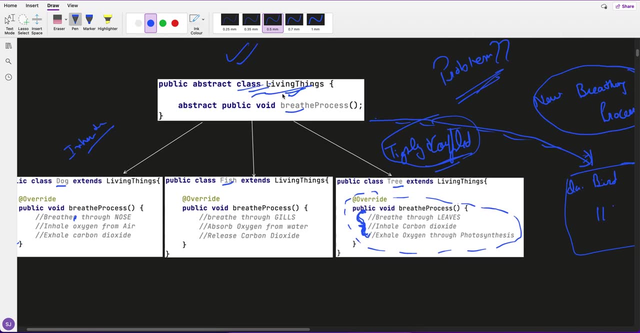 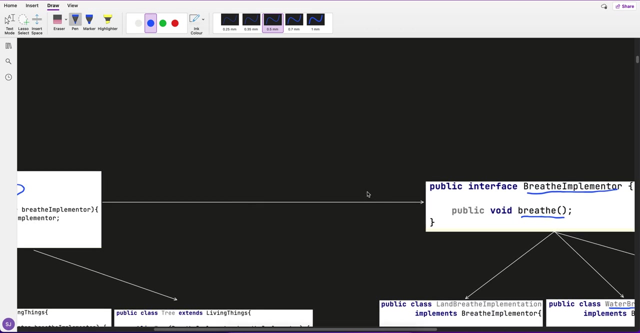 carbon dioxide. similarly, i have given one child class or tree: breathe through leaves, inhale carbon dioxide, exhale oxygen. right now, here, what i have done is in the previous abstract class living thing. what i have done is i have a reference of this implementer. i have a reference. 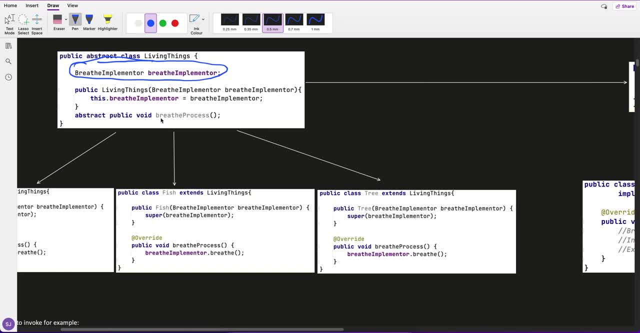 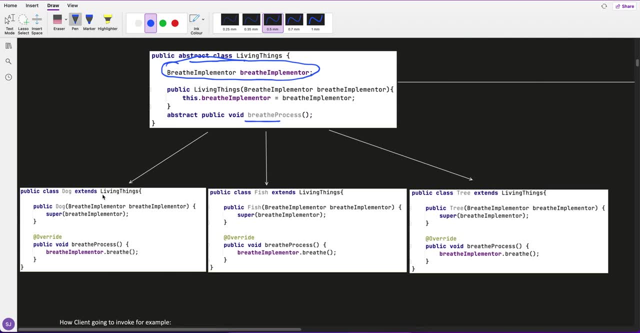 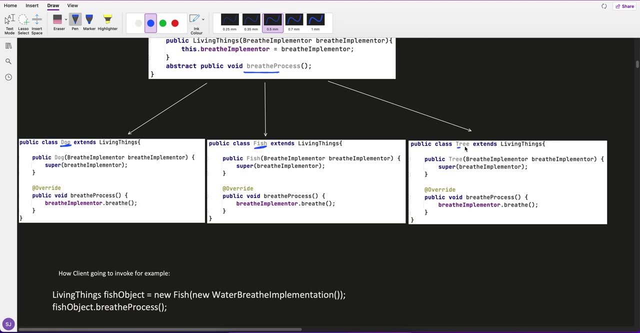 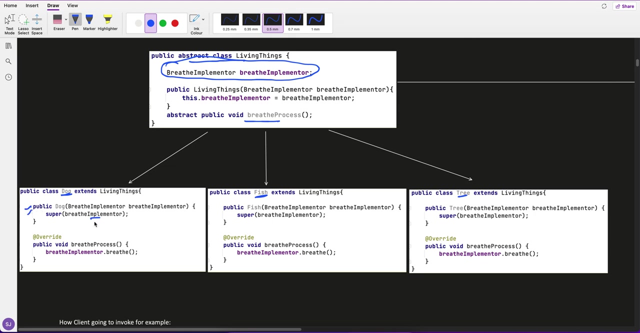 of this implementer. right now, again i have the same method: breathe process. right here i have a process breathe process. now it's child class dog, same dog fish tree. so i have also have a child class dog fish tree. but here now see the difference. you now in the dog constructor, it is passing. the breathe implementer: it wanted fish, it is passing. 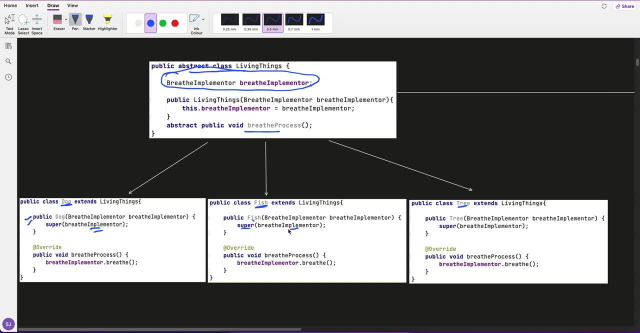 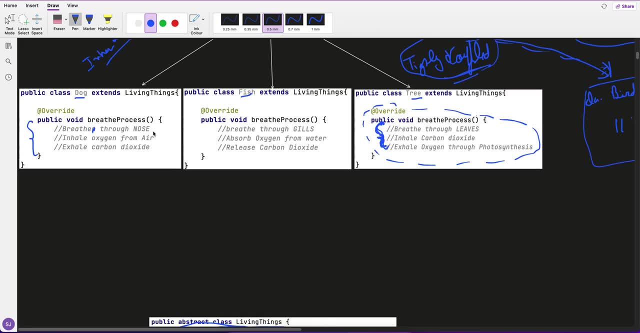 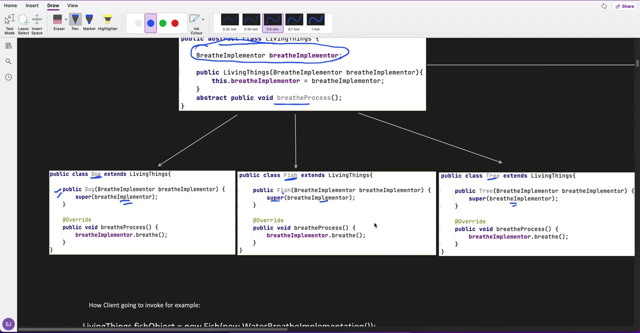 to its parent. what is the breathe implementer it wanted. similarly, tree, it passes to its parent what is the breathe implementer it wanted? and in the breathe process. earlier we were having all this logic here, but now we have separated this logic into the separate classes here in the 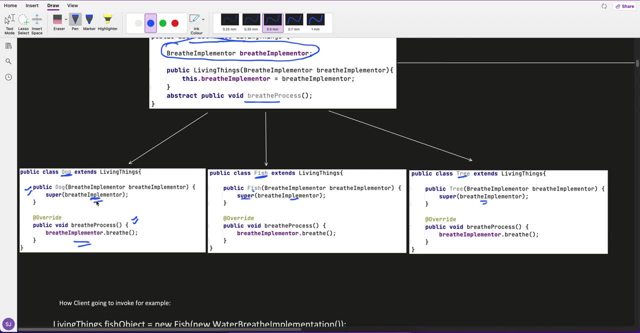 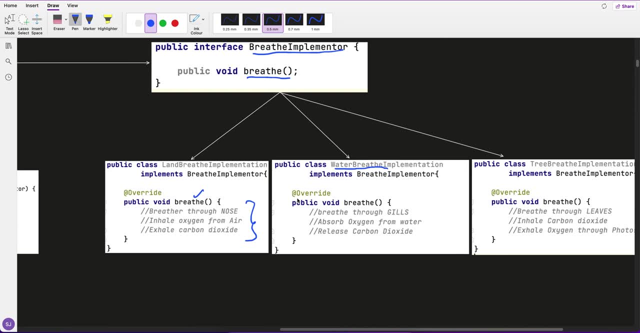 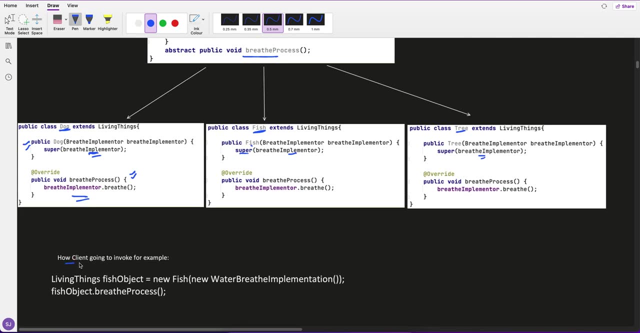 process. now we are just doing breathe implementer. bite the implementer. whatever the implementer would be call its breathe method, whether, if it's using land, breathe implementer, it will call this method. if it is using water, breathe implementer, it will call this method. right. so here, if you see that, if how the 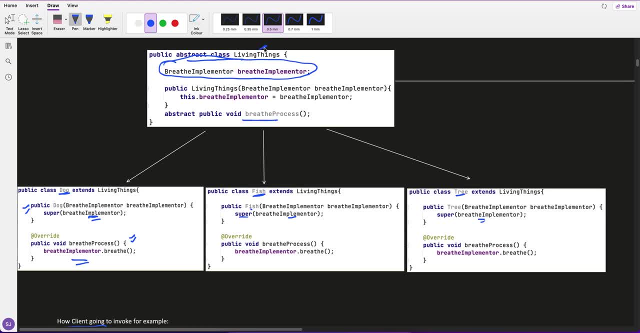 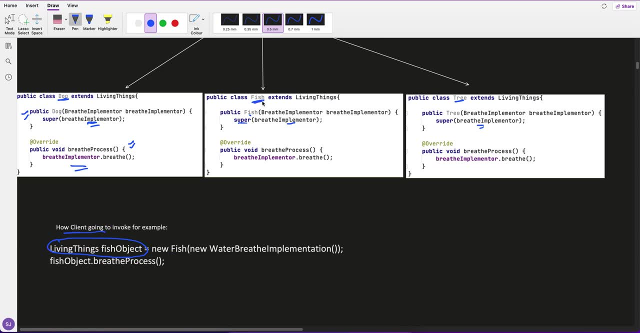 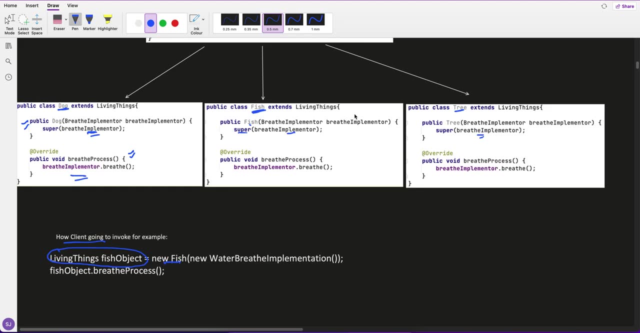 client will invoke this, so it will create an object of this living thing. so, living thing, let's say, i am creating a fish object- new fish. i am creating this golf object- new fish- and putting into its parent living thing. and what is the breathe implementer? I am passing, I am passing a water breathe. 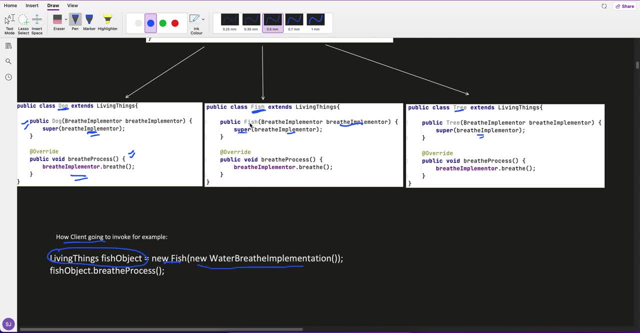 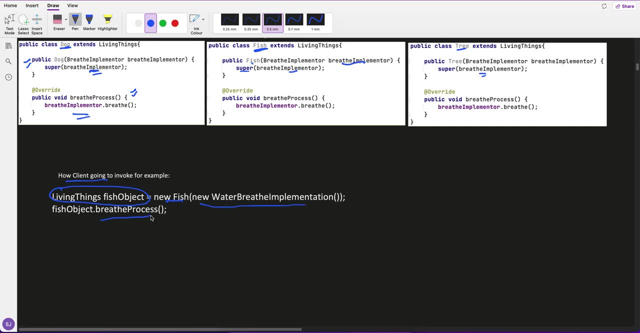 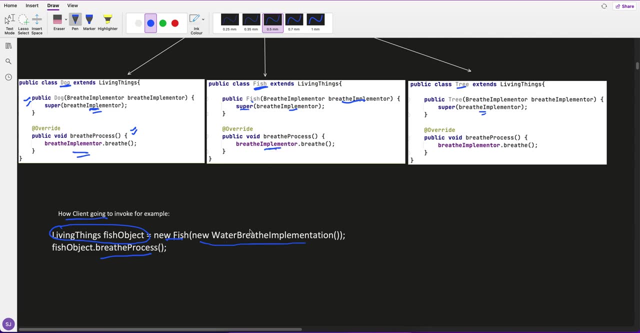 implementer to it: water breathe implementer. so this method will call water breathe implementer. will be set here right, and when I call breathe process, fishbreathe process, it will call breathe implementer. now, what is the breathe implementer? this one water, it breathes. so 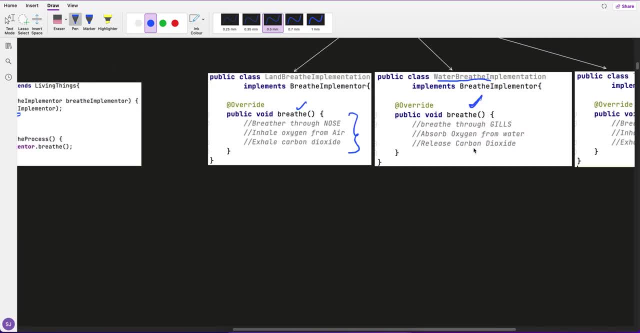 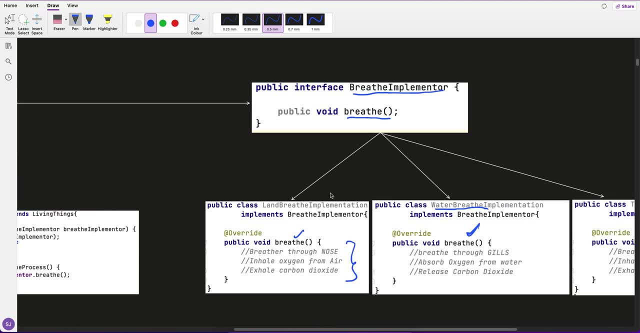 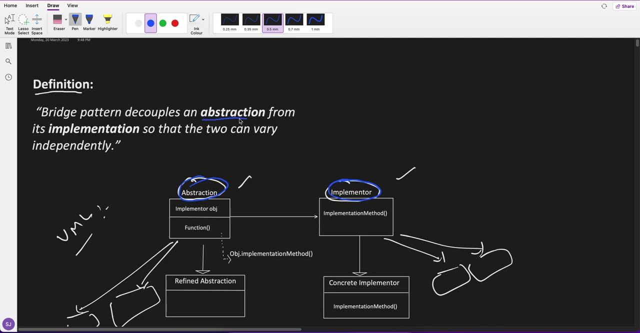 So it will call waterBreatheImplementedbreathe this one. So now, what is the advantage of this? Now, the same part we have divided into like this: Now, what is the advantage? So, advantage is what is? it decouples an abstraction from its implementation, so that 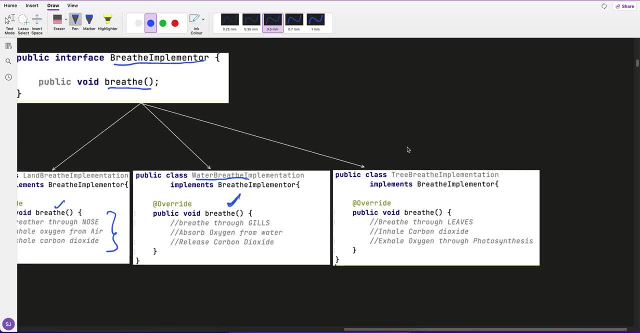 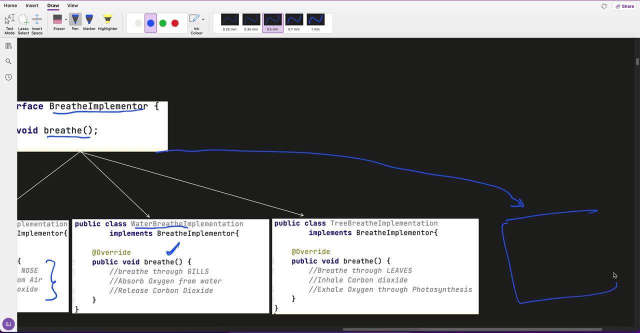 two can vary independently. Now here, let's say: in future I need to add one more breathing process. I can add it simply. I can add it simply. let's say, breathing process of something. let's say public another XYZ breathe implementation. 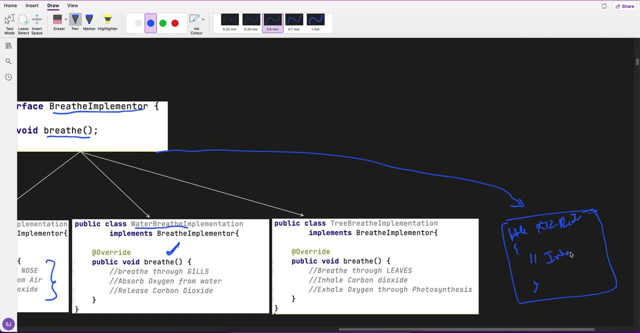 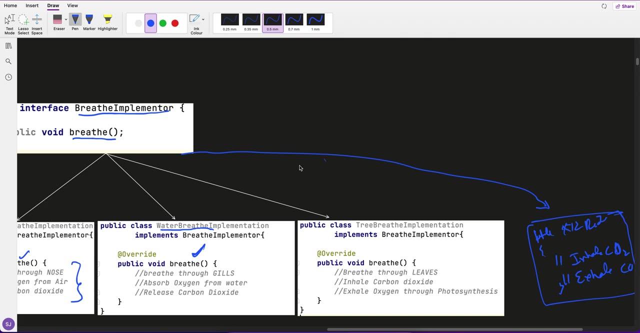 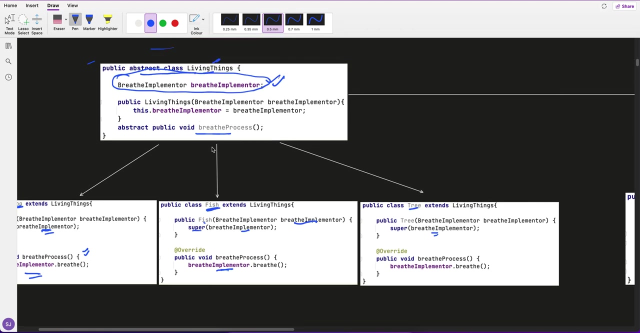 I can add its new breathing process like: inhale carbon dioxide and exhale carbon dioxide, So it's a total different breathing process. So I So it can vary independently of abstraction, even though abstraction is abstraction. If you see that this one is nothing changed, even there is no child class which is using. 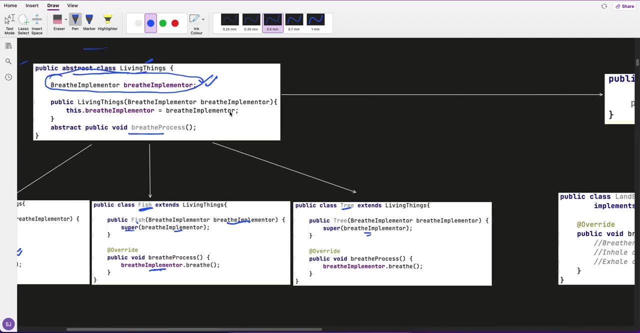 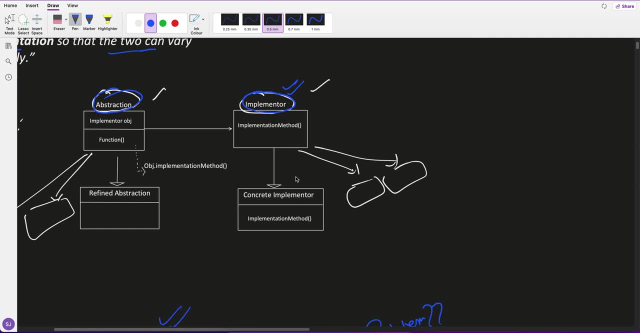 this, but still it can grow, It can vary from its abstract. this thing right. So that's why this is UML. So you have an implementer- it's concrete. you have an abstraction- it's concrete. and here it has a reference of implementation. 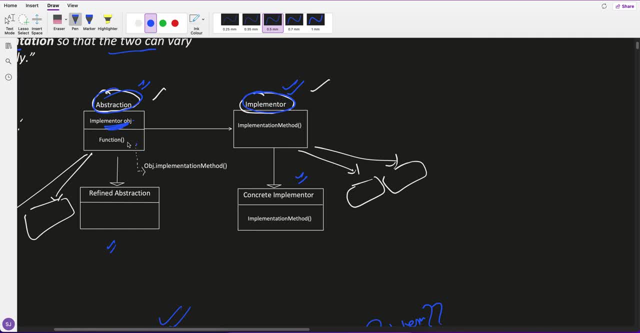 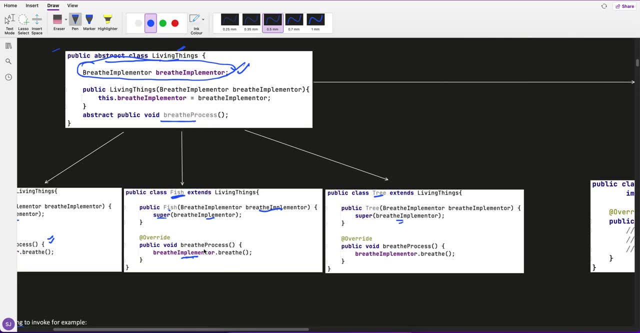 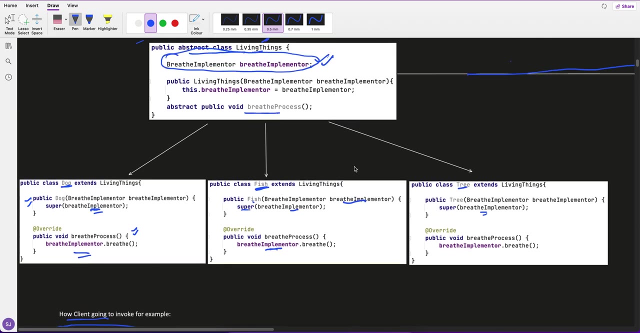 Okay, And here, in the function which it has, it ultimately invokes- it's this methods, right? So you understood this bridge. So this is nothing but a. you can say that it is considered as a bridge, right? Similarly, let's say for tree: what will happen? 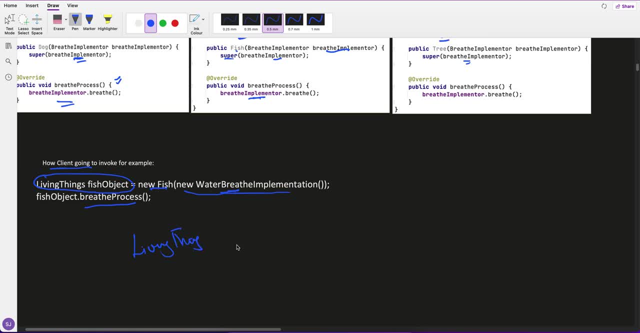 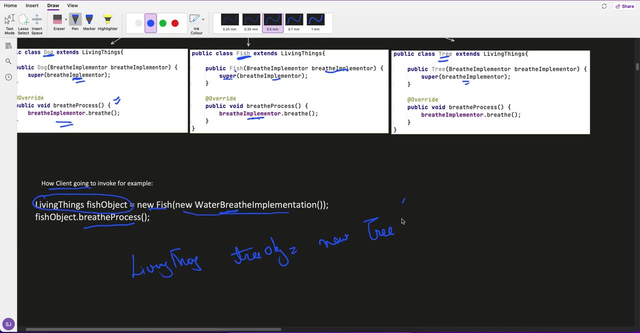 So let's say living thing. let's say I'm creating a tree object equals to new tree. Okay, Okay, Okay, Okay. And let's say I want to give it a capability of a land, water tree or this. so I let's. 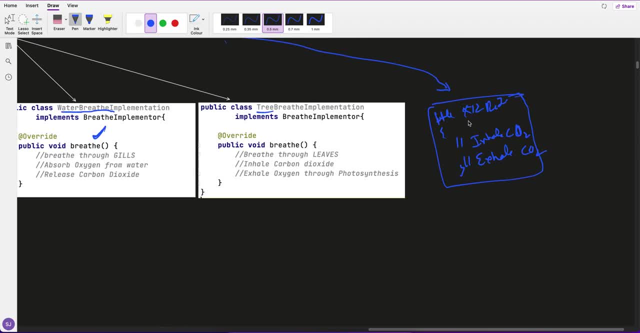 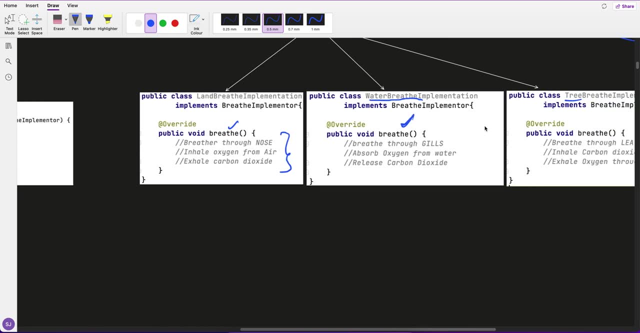 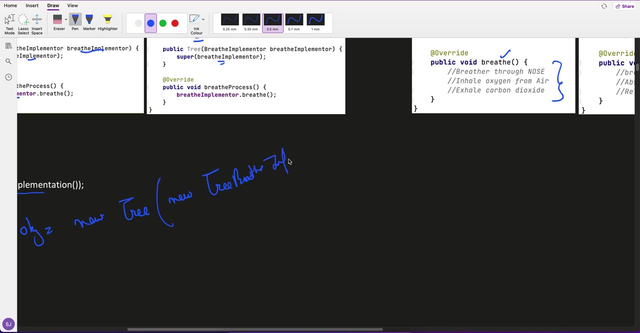 say I want to give it a tree right Sometime. let's say yeah, tree breath implementer, give. let's say new, I'm giving a this one. new tree breath implementation, new tree breath implementation, I'm giving it. 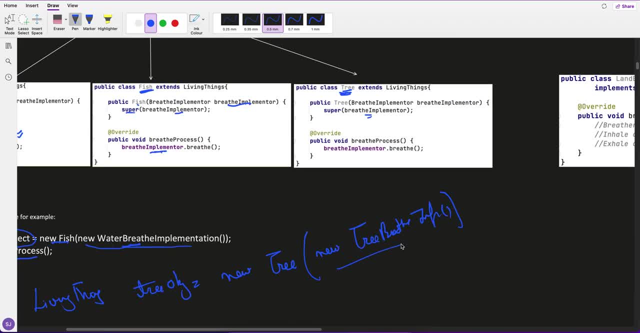 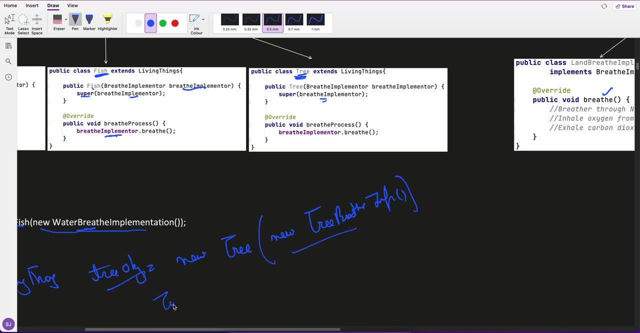 Okay. So now here, if you see that the tree object, Okay, I'm passing three, breathe implementation, I'm passing this one, right. And when I'm calling this object, three object dot. three object: dot, breathe process, breathe process, what it will call breathe implementer. 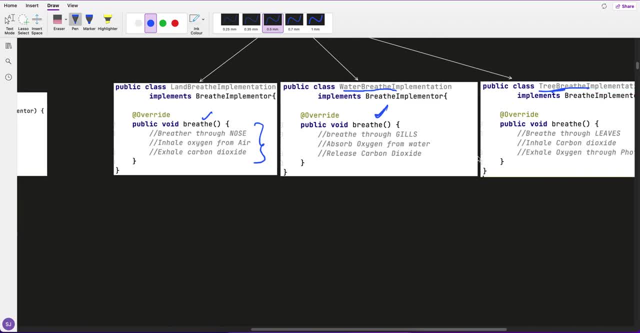 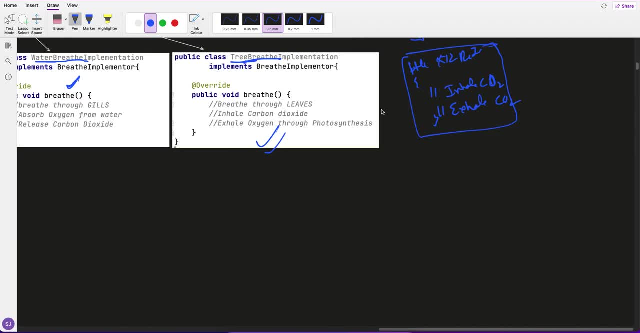 This is the breathe implementer, right. Tree B, dot B. So this will get involved, right. So now just see this, even for tree. If I want this, the new one, Okay. X Y, Z, certain, which is added: inhale CO2 and exhale CO2, inhale carbon dioxide exhale. 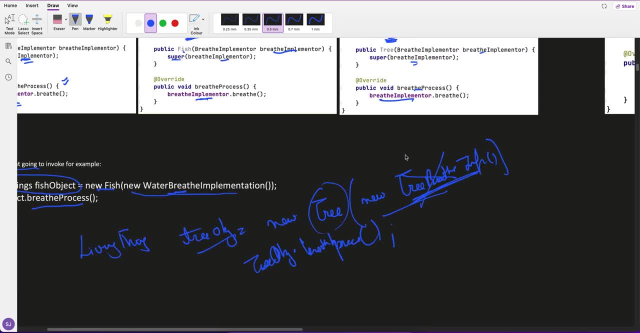 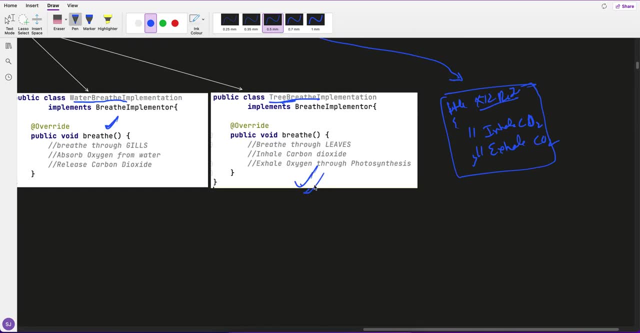 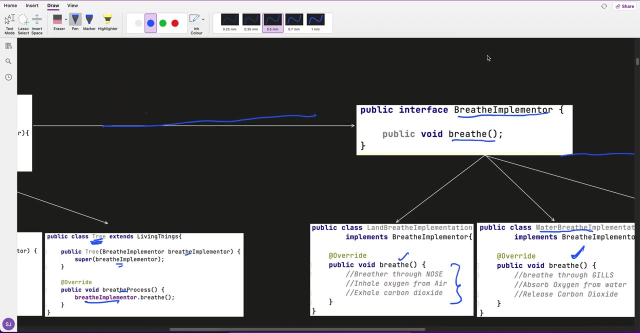 carbon dioxide. I can change it on the run time. Let's say I can give X, Y, Z. uh, what is that? breathe implementer. So it will call this now. So now here. this is a problem. breathe, a bridge pattern. solve that both. implementer and abstractor. 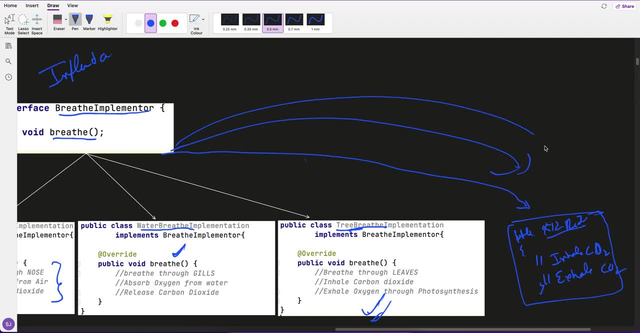 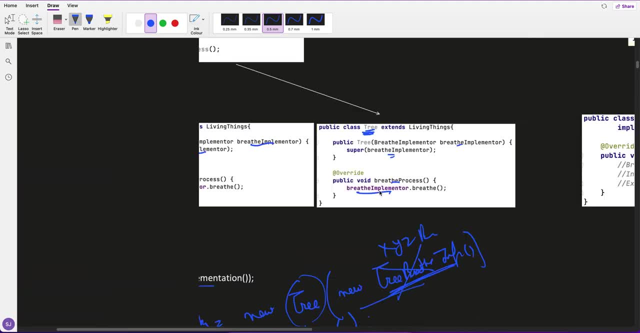 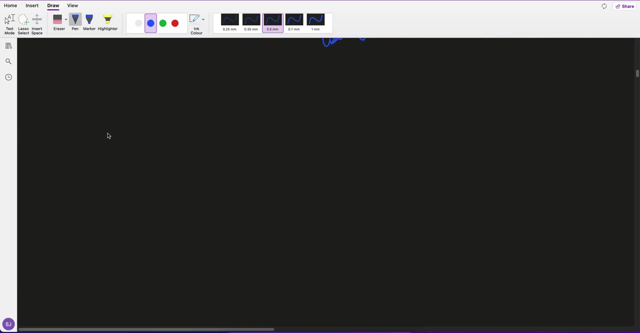 can vary independently. This can grow. This can grow independently of the each other. Okay, Got it. So this is the one. but now you might. if you have gone through strategy pattern, right, You might now strike till now. Hey, isn't it very similar to strategy? 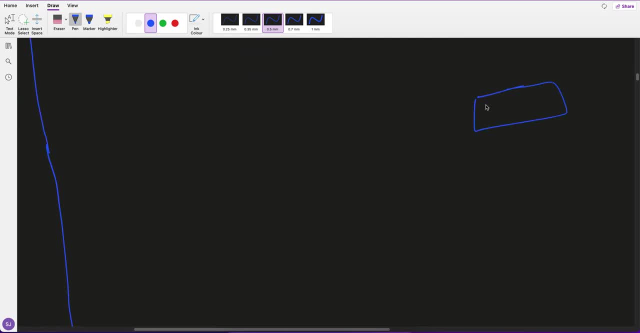 So this is the strategy pattern. So here, if you see that it has a strategy, Okay, Okay, So I can create a breathing Okay. So here, if I click this interface, let's say I created the same example, Let's say I have creating a breathing strategy, breathing strategy. 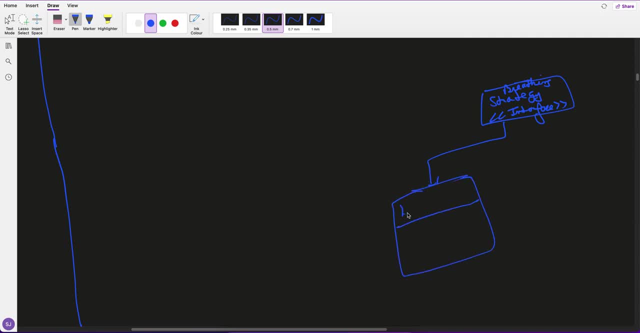 I can have a different, let's say, land breathe strategy. Similarly, I can have water Breathe- Can you see this, Yeah, strategy. and one more I can have is tree breathe strategy, and similarly I can have more right. this strategy is used by one context class which has this strategy object: strategy object. 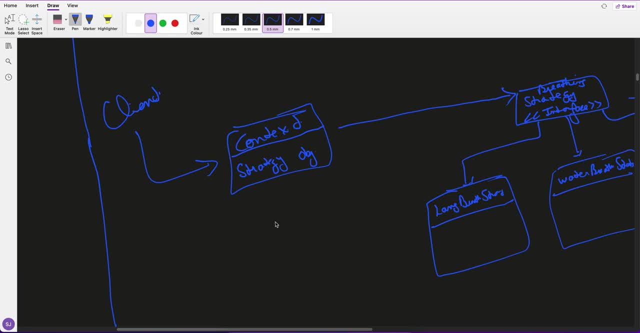 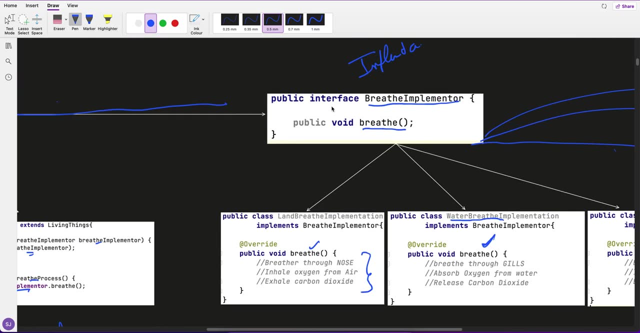 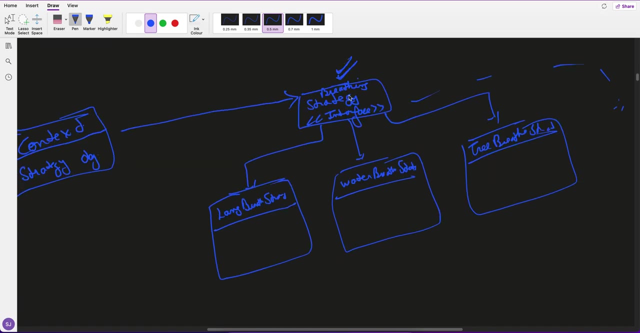 and clients use this right. so now here, if you see that it is very, very similar to what we have here, we call an implementer nothing, it's in the strategy, it's nothing but a strategy. we call it strategy interface and we have this right. so here we have land breathe strategy. 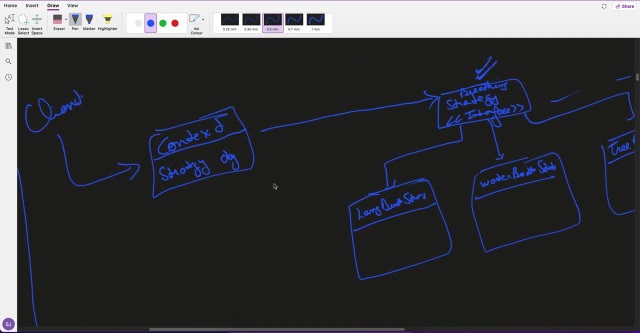 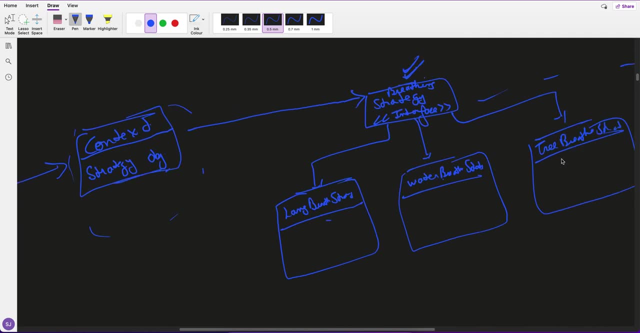 water, breathe strategy, tree based strategy. so, and here it's a concrete where it has an object of it's strategy right Which can have either land, water or tree right, and it has one function that will just call that, whatever the object dot, let's say breathe, and it has breathe method, it has breathe method. 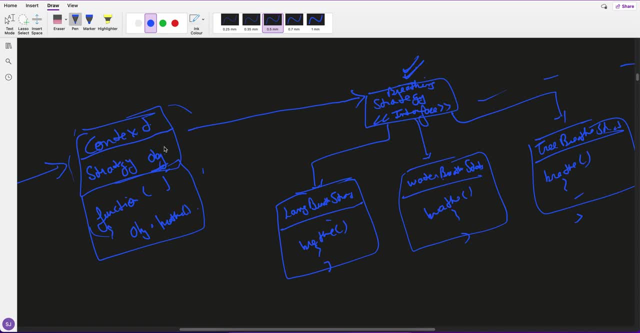 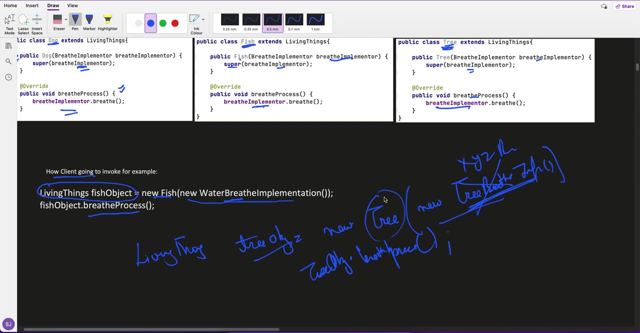 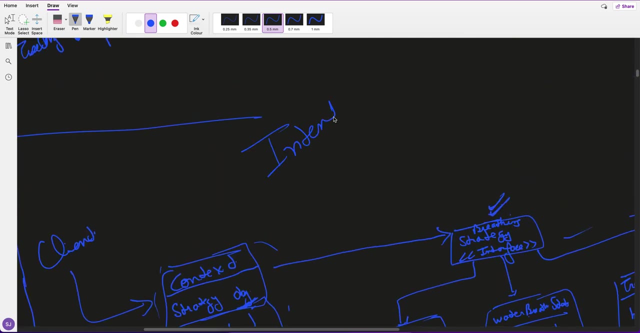 breathe method. so it calls object dot breathe. so now, whatever the object you have said, it will call it. So this is exactly same as breathe Bridge pattern. now, how is the different like? now, the difference is only on the intent. so see in, you will learn so many design patterns and lot of design patterns are very similar. 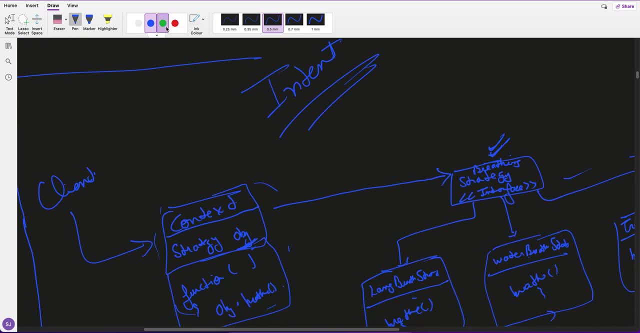 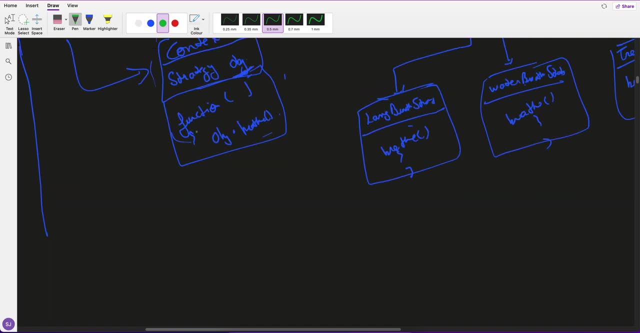 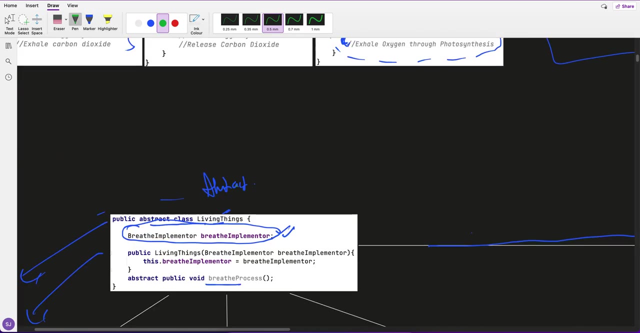 but difference in the intent. so you have to understand the intent of what is the intent of a strategy pattern. so the intent of strategy pattern is that change the behavior of this object which it called context. Here in the bridge it call as abstract class. so in the intent of the strategy pattern it's. 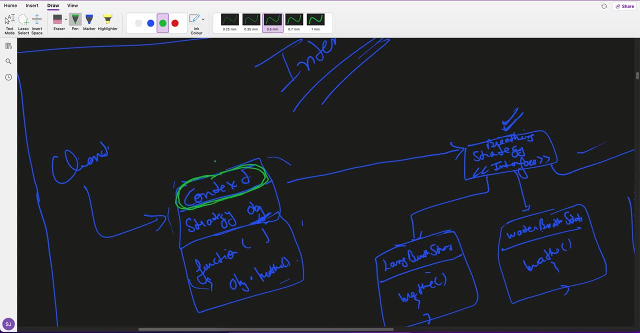 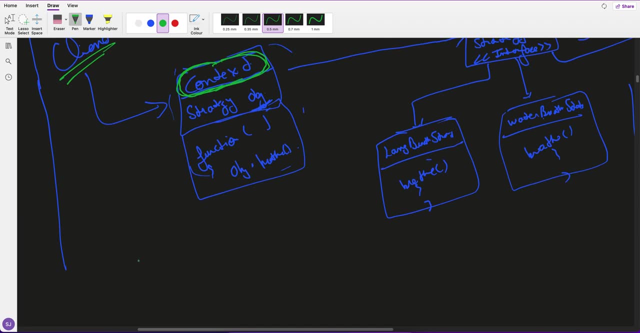 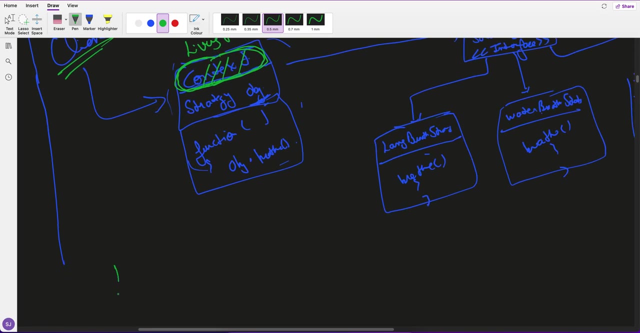 intent is to change the behavior of this object on runtime. let's say, for example, client, clients create an object of. let's say this context, right, let's say I will call this context as the living thing on itself, living thing which we are creating. so let's say it's creating. 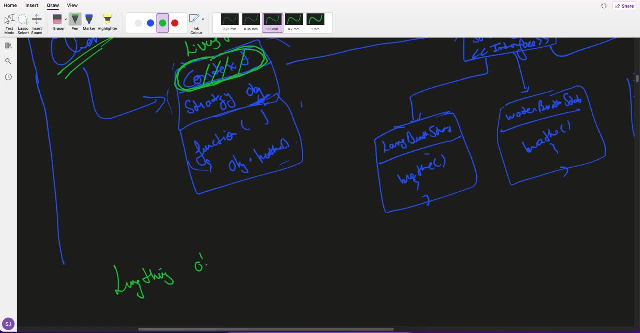 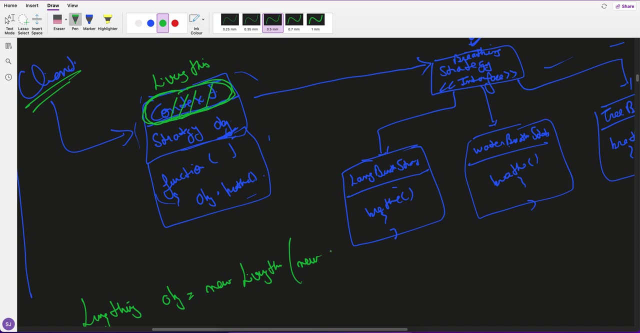 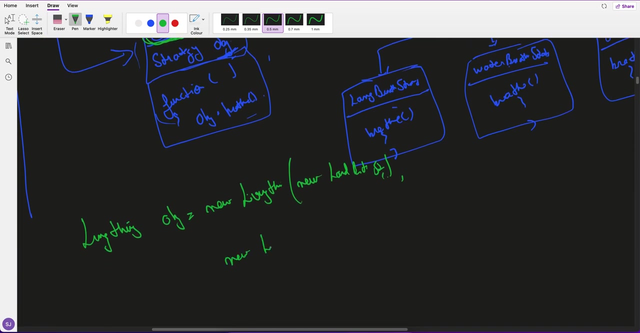 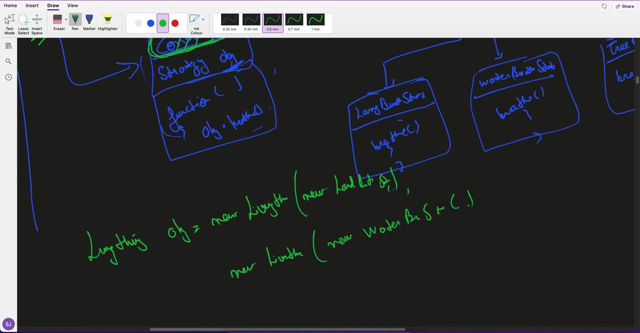 an object of this thing- living thing- right. Object Equals to new living thing. now, let's say it has a constructor where it. I'll pass the strategy object. it can pass land- new land, breathe strategy. or it can also pass living thing- new water, breathe water, breathe strategy right. 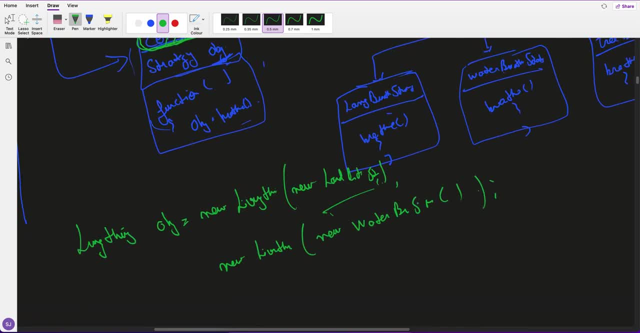 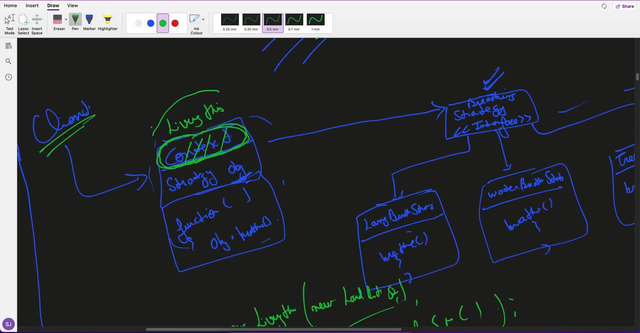 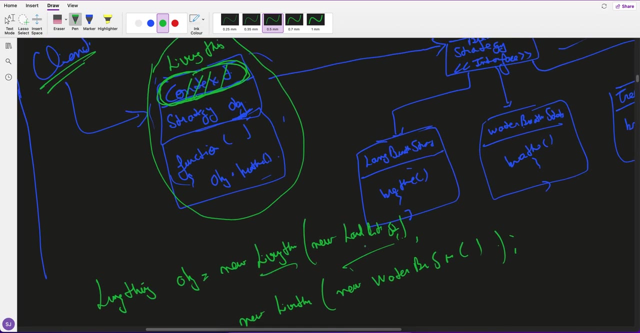 So It can change anything either land breathe, water breathe into the same object. so the intent of the strategy is to change the behavior of this object dynamically on runtime right. so currently, if you see that for this living thing object, it pass the land breathe object. so when this method will call it, change the behavior of this one object. 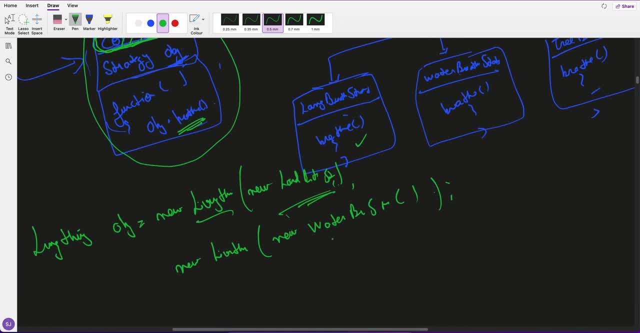 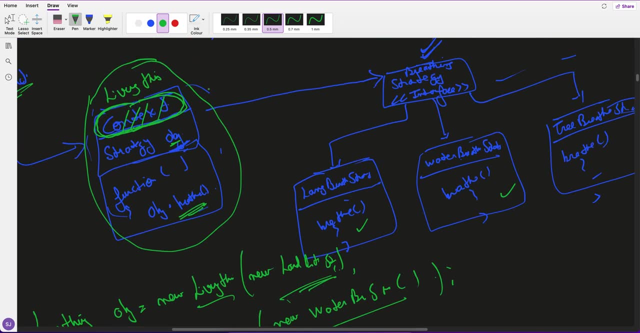 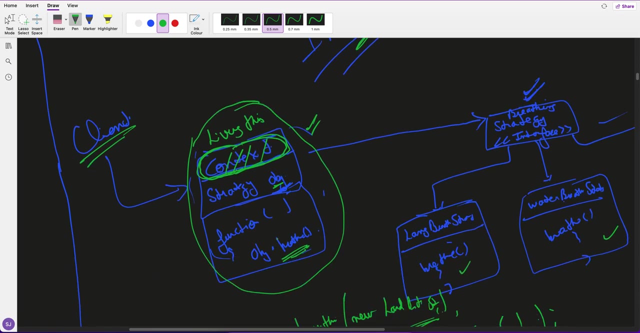 Breathe, so it will call this breathe. now it pass water breathe strategy into this one. so when you call object Breathe, it call this. so you are changing the behavior of this object on runtime. which one will you pass? But what is the intent of bridge pattern? the intent of the bridge pattern is that if this: 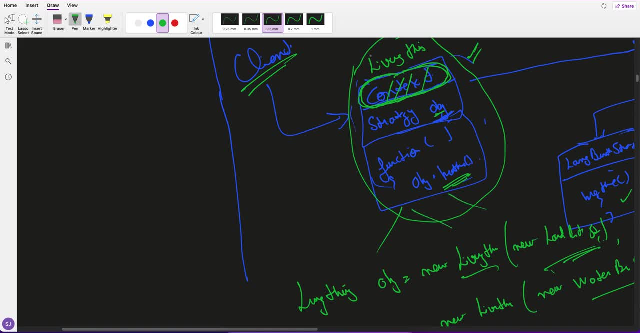 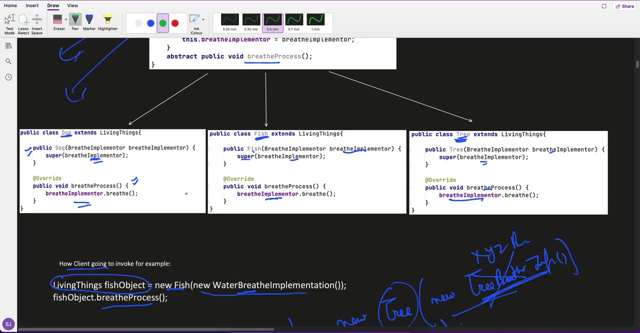 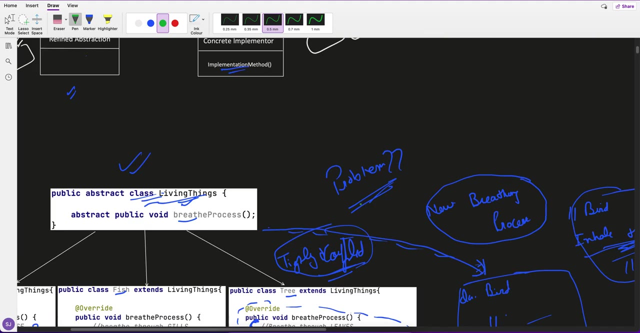 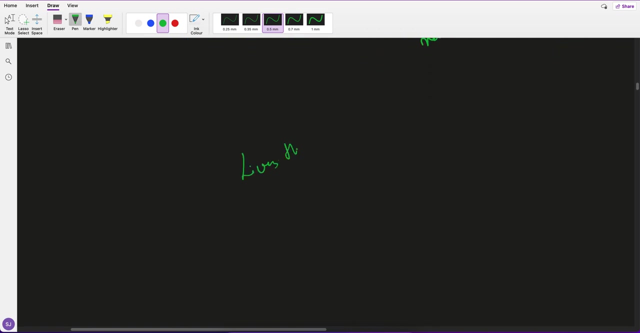 class grows. let's say now, this is change it to abstract, right, change it to abstract and this class grows. now, bridge pattern intent is that both should grow independently, Right? So Let's say: if this class grows, this class grows. let's say: it has only living thing currently. 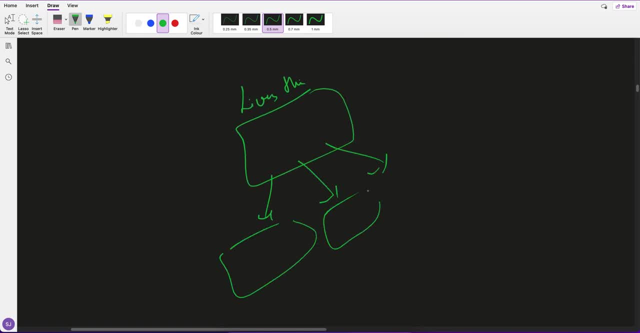 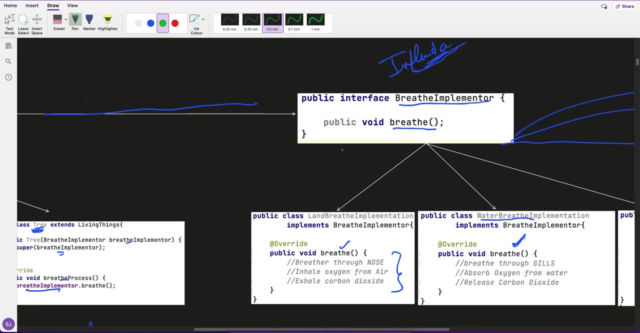 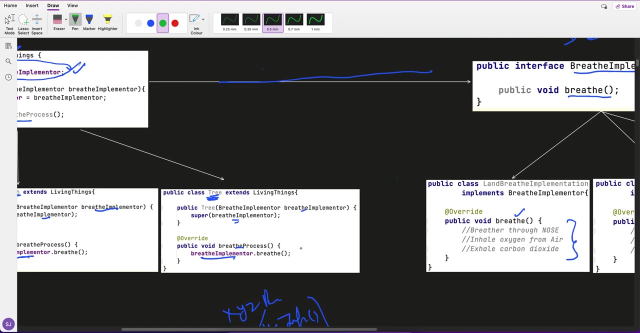 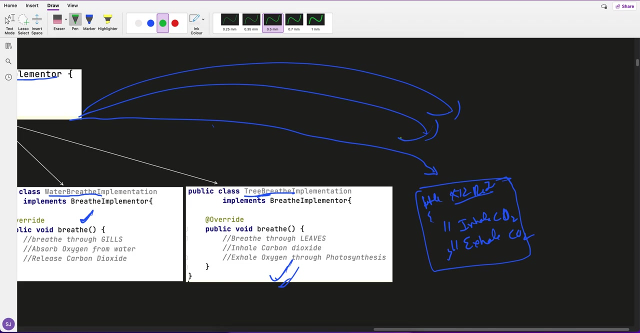 but now, in future, if this class grows and it has certain methods, divided like how we divided it, like into an implementer, So bridge pattern is designed from that perceptive. separate the logic, whatever the logic you have, So that both can vary independently, both can increase, decrease independently, but somehow